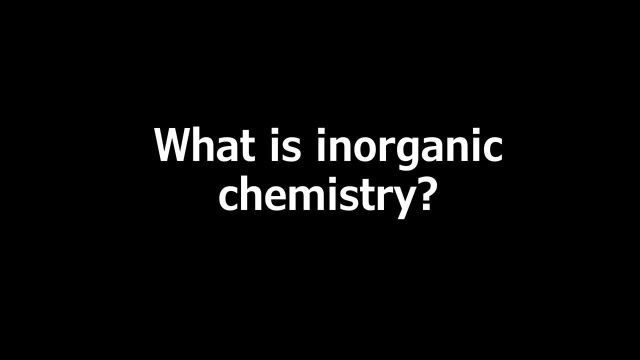 What is inorganic chemistry? To answer this question, we need to delve deeper into its precise definition. While organic chemistry is centred around carbon-based compounds, inorganic chemistry focuses on non-carbon-based compounds. However, this definition can be a bit. 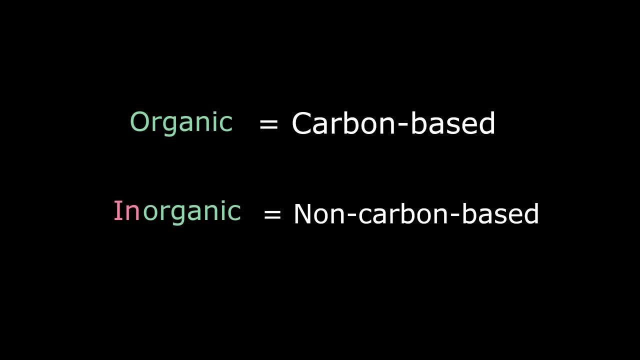 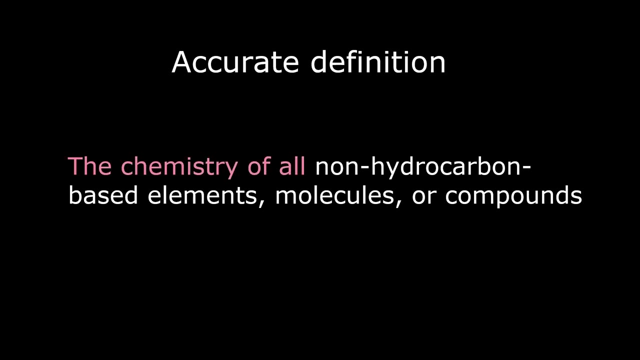 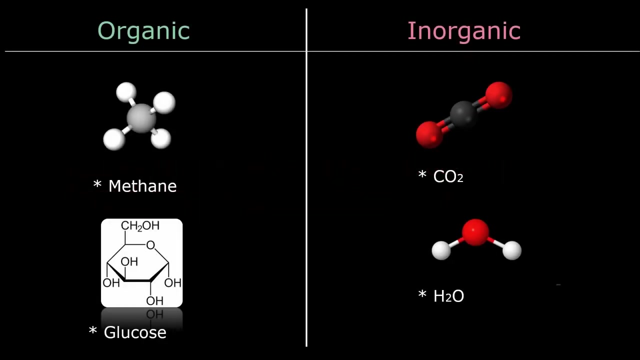 confusing because certain compounds, such as carbon dioxide, are considered inorganic despite containing carbon. To avoid this confusion, a more accurate definition is that inorganic chemistry is the chemistry of all non-hydrocarbon-based elements, molecules or compounds. Therefore, we can classify compounds like methane and glucose as organic, while water 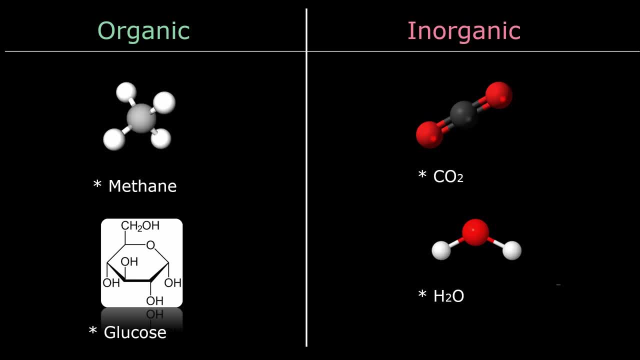 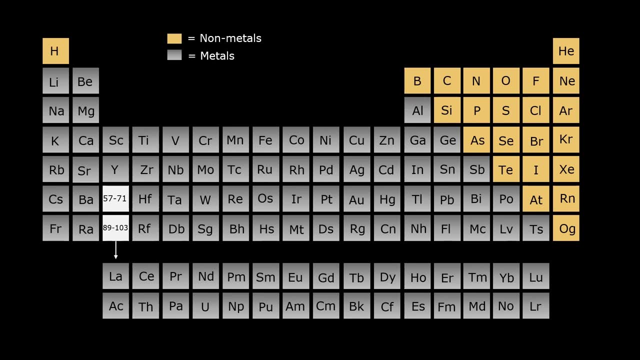 and carbon dioxide fall into the category of inorganic Compounds. Now let's take a look at the periodic table to better understand the scope of inorganic chemistry. Carbon being a non-metal, predominantly forms bonds with other non-metals like oxygen. 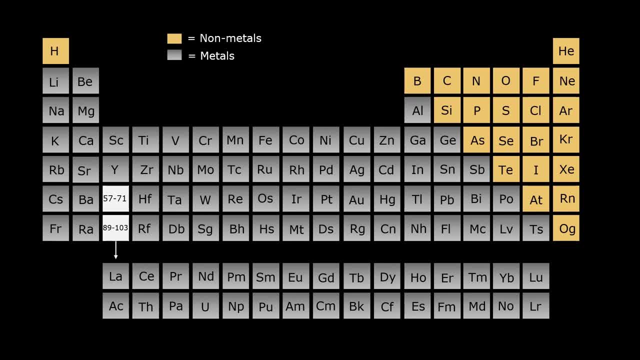 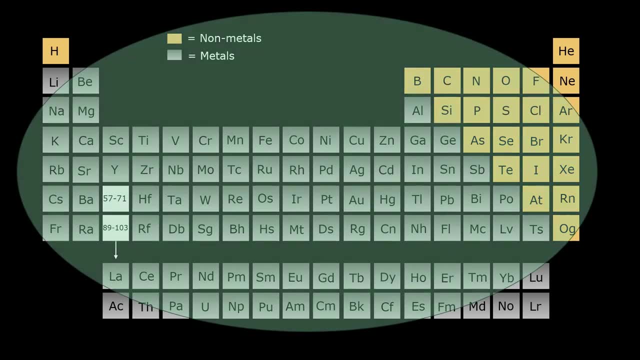 nitrogen and other carbon atoms. This is why organic chemistry primarily focuses on this specific region of the periodic table. In contrast, inorganic chemistry encompasses the entire periodic table, including non-metals and metals. In this sense, inorganic chemistry serves as an expansion of organic chemistry. 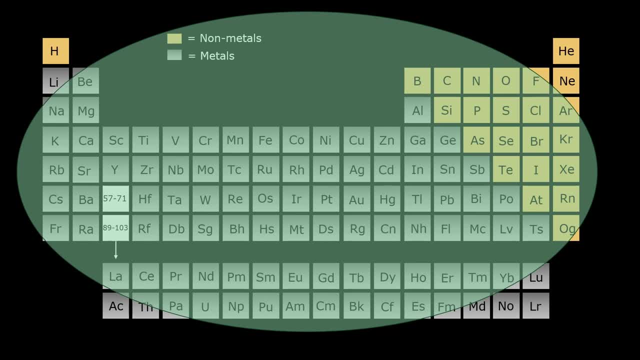 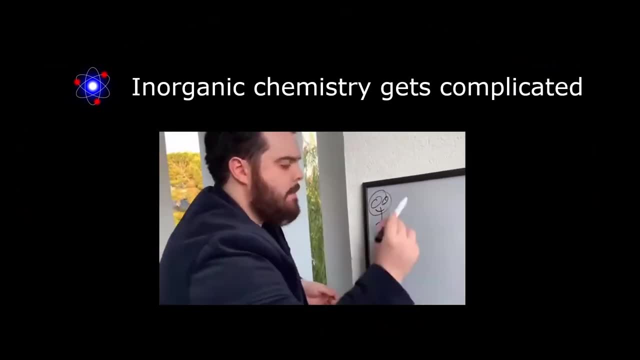 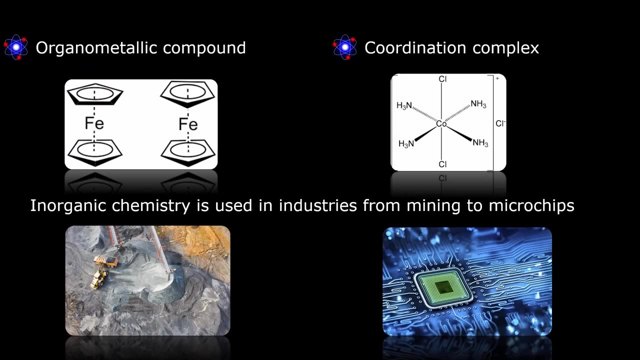 broadening its scope to encompass all elements. As a consequence, inorganic chemistry becomes increasingly complex due to its inclusion of all the elements and their distinct properties. Conclusion: This results in the realm of inorganic chemistry having many fascinating subfields of study, such as organometallic compounds and coordination complexes. So inorganic chemists end up finding: 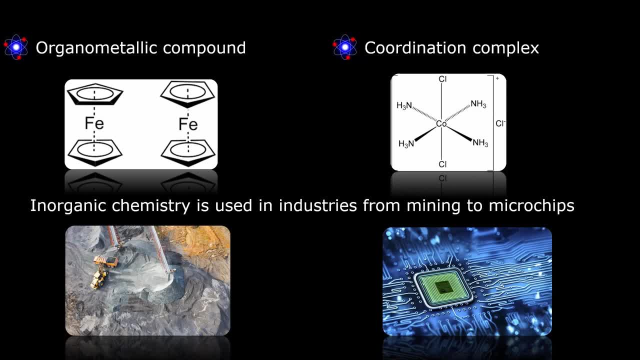 employment across a wide range of industries, from mining to microchips. As mentioned before, inorganic chemistry is not solely concerned with studying elements and compounds. it also explores physical principles. So you might be wondering: what do these compounds do, how do they behave and what are the underlying principles governing their behaviour?